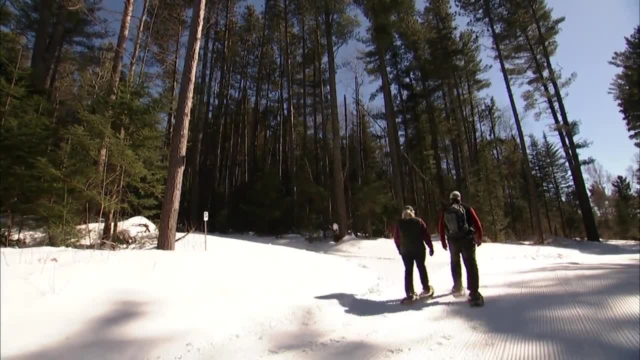 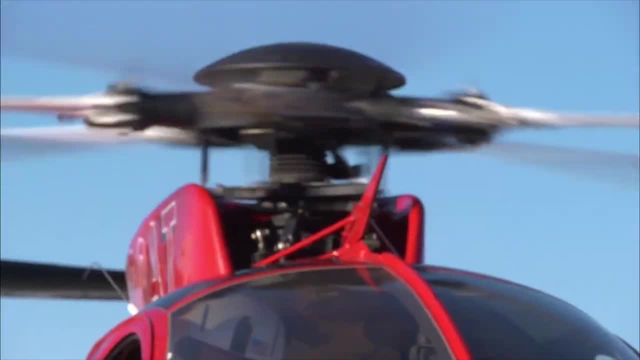 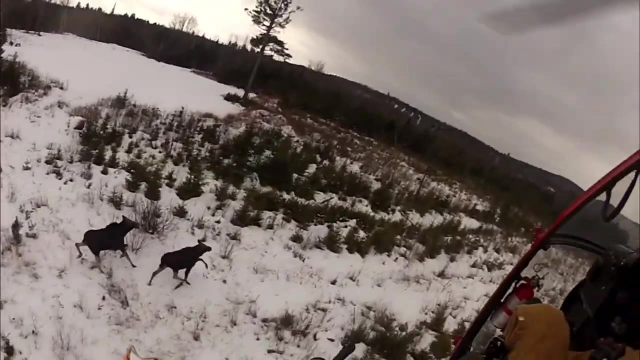 We're getting funny signals on HARI SREENIVASAN. Scientists are bundling up and prowling the forest in pursuit of the largest wild animal in New Hampshire, the moose. Their into-the-woods exploration by both foot and air is part of a massive research effort to understand why America's iconic 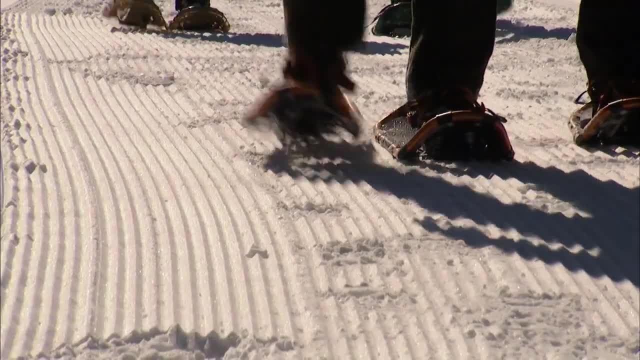 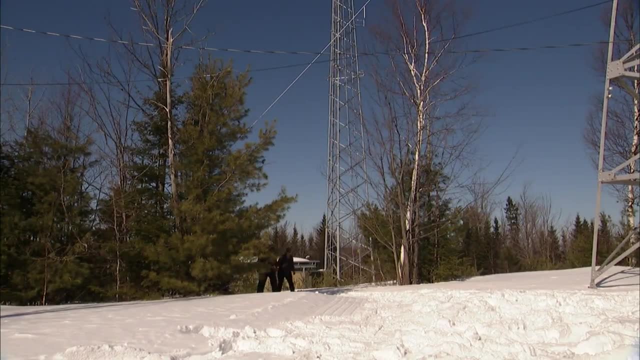 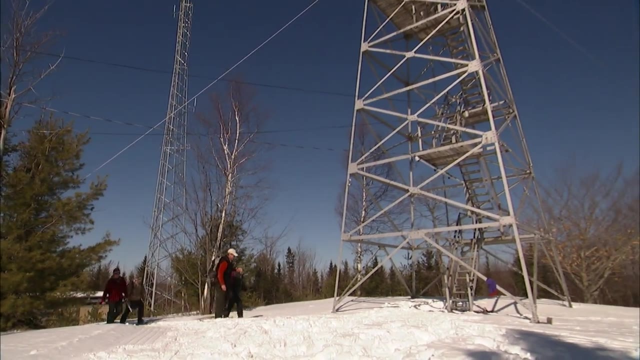 wild moose are so important, They are dying at alarming rates. The first weeks after a long winter are a critical time for moose, And here in New Hampshire wildlife biologists from the state Fish and Game Department want to find out why, in the last three years, moose populations are down as much as 40 percent. 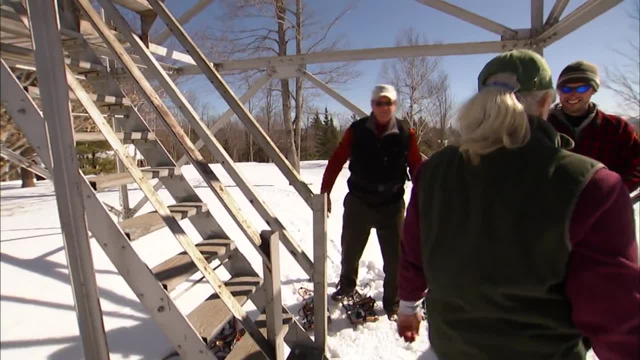 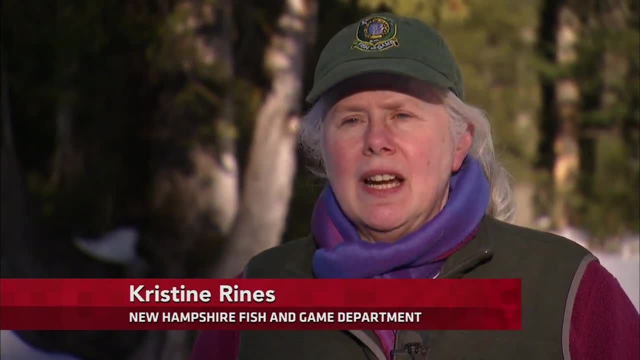 in some regions. Christine Rines is the moose project leader with New Hampshire Game and Fish Department. CHRISTINE RINES, Moose Project Leader, New Hampshire Game and Fish Department. April is the month of death. when most of these animals seem to just, they are completely. 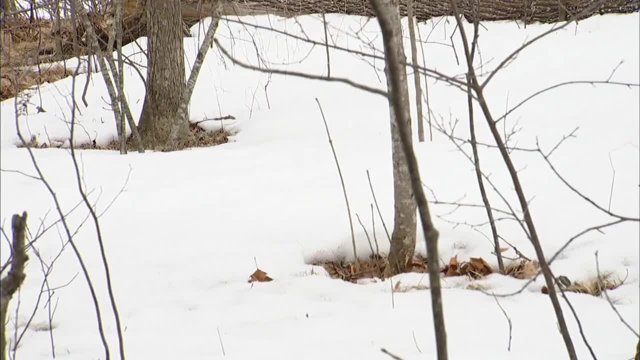 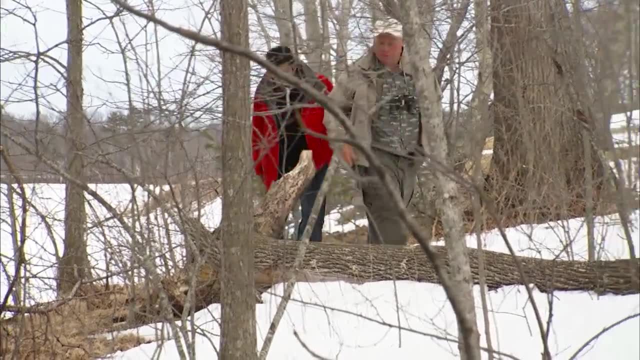 depleted and they just start dying. HARI SREENIVASAN. According to Eric Orff, New Hampshire field biologist for the National Wildlife Federation, the deaths have been dramatic all along North America's southern moose range. ERIC ORFF, New Hampshire Game and Fish Department. 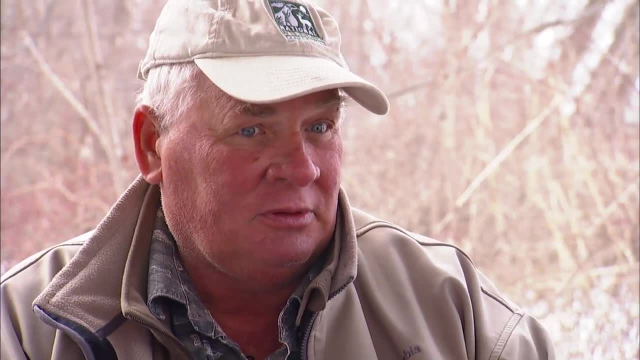 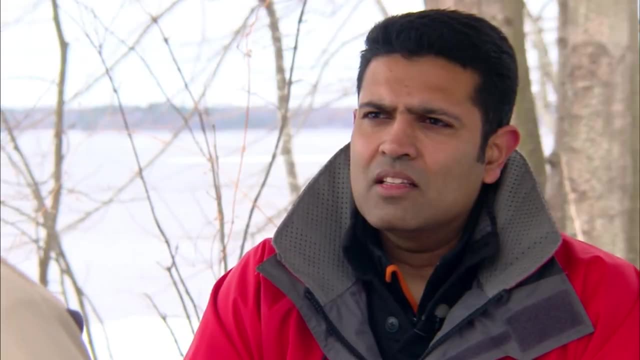 When you look at a precipitous decline in the last decade, you know the needle is headed in the wrong direction. You know, all across the southern edge of their range, from Nova Scotia, New Brunswick, Minnesota, Michigan, all across the southern fringe of their range. 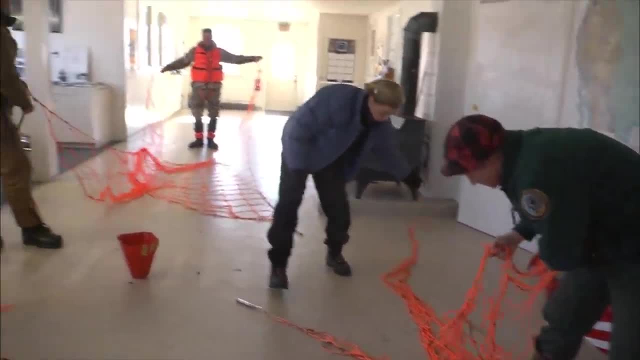 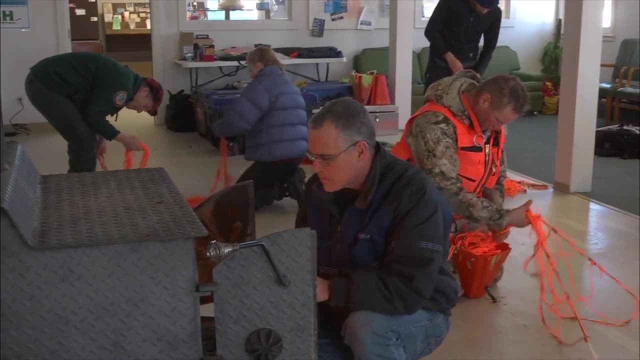 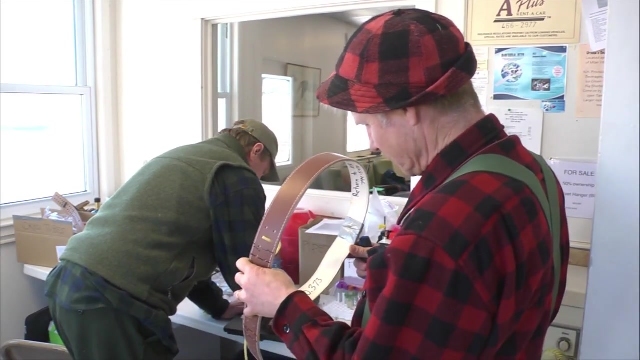 numbers are in a significant decline. To better understand what's behind the decline, New Hampshire and Maine have hired capture teams whose job it is to track down the moose and collar them with a radio transmitter. All right, well, we need the radio frequency at 150- 373.. Pete Peekins, professor of wildlife. 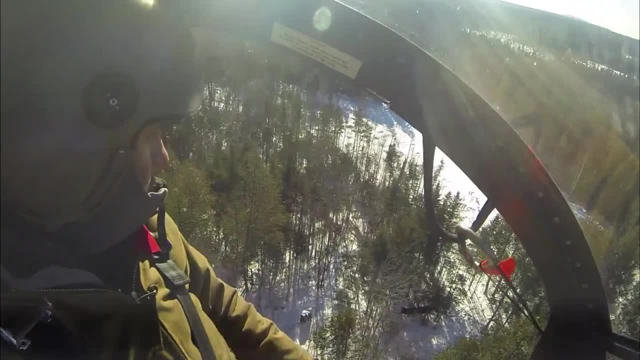 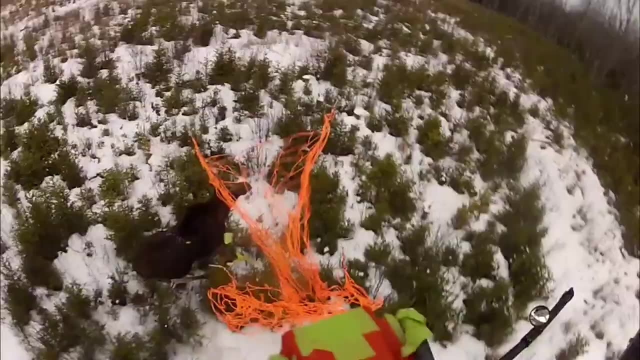 ecology at the University of New Hampshire is overseeing the project. The helicopter basically finds these animals, zooms down on that animal, a net is shot over the gun- we call it net gunning- and the animal trips up in the net. and what? 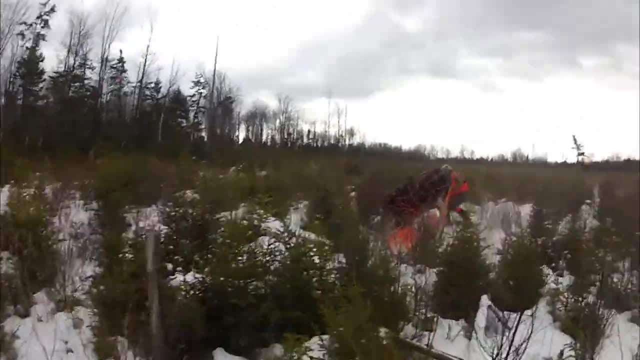 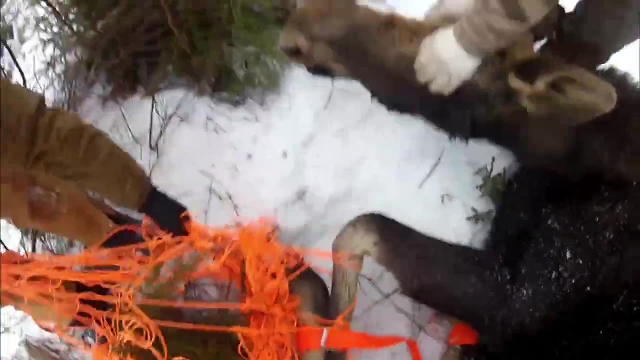 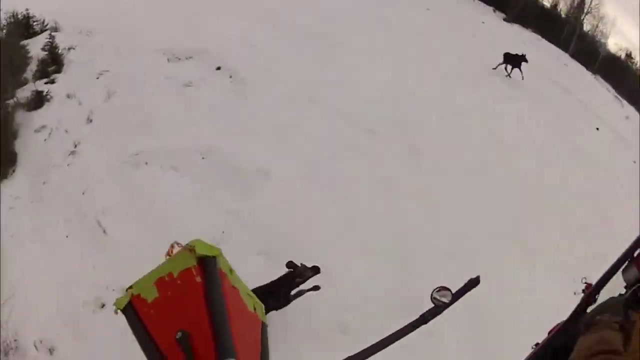 are called muggers, jump out of the helicopter at low, low height and they wrassle the moose to the ground. and the people we use- actually many of them- have been professional rodeo cowboys. The goal is to collar and release 200 moose. 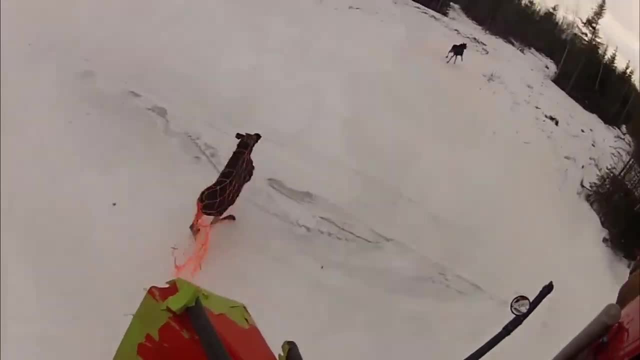 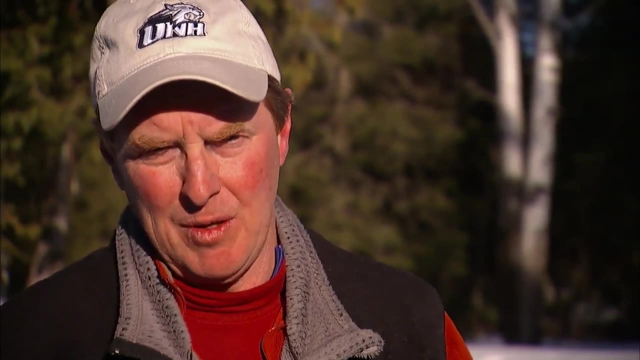 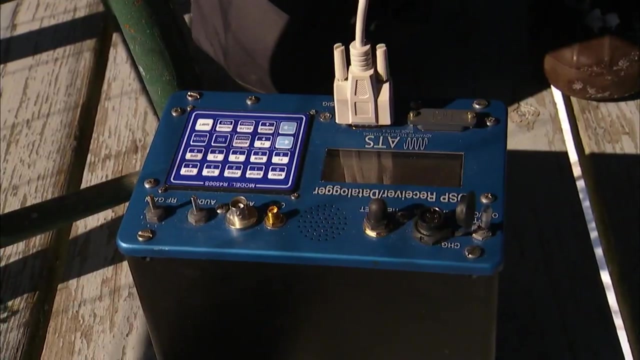 between this winter and next. you, These people, know how to handle big animals, Most importantly to us, how to humanely handle an animal. Professor Peekins' team tracks the collared animals from a fire tower in northern New Hampshire. Each day devices are checked. 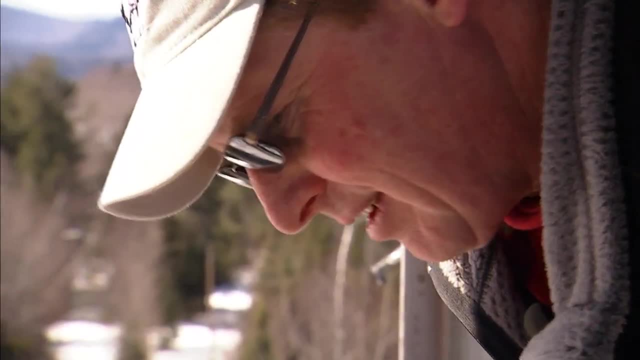 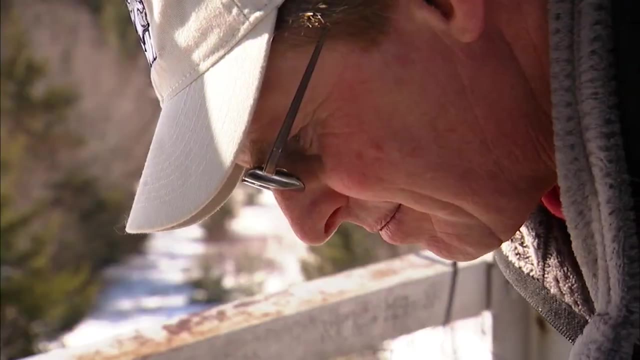 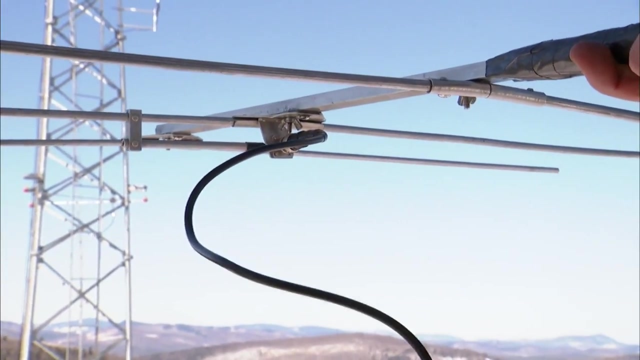 for signs of life. Of the 40 moose out there, how many have we successfully monitored here today? So we picked up 37 of the 40. And from this morning there's one 314, if you want to check that one, Nick. 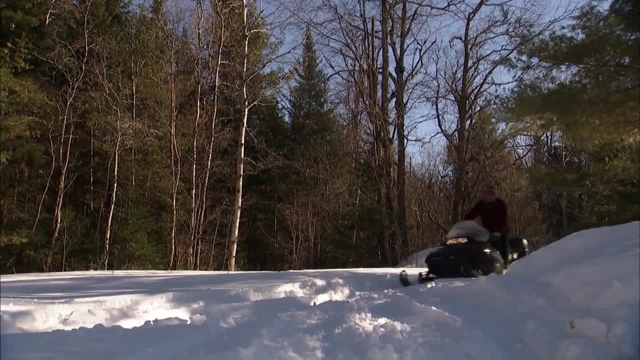 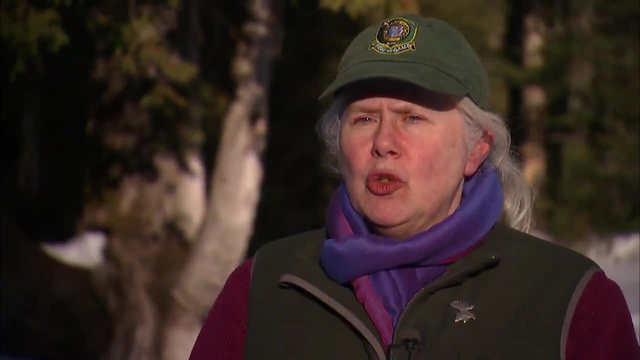 When monitors signal a moose death, researchers are quick to get to the animal before vital information is diluted by weather and time. What we're going to try and do is get to them much sooner, so that we have better information on exactly why they're dying. 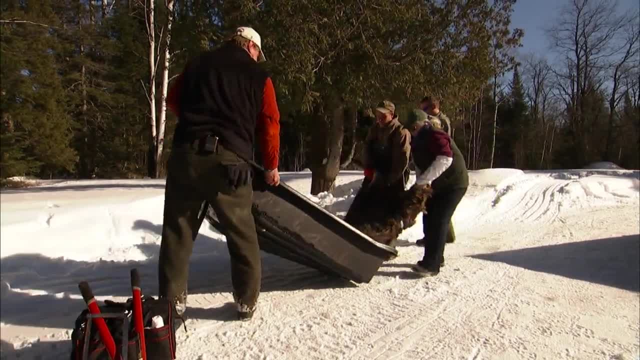 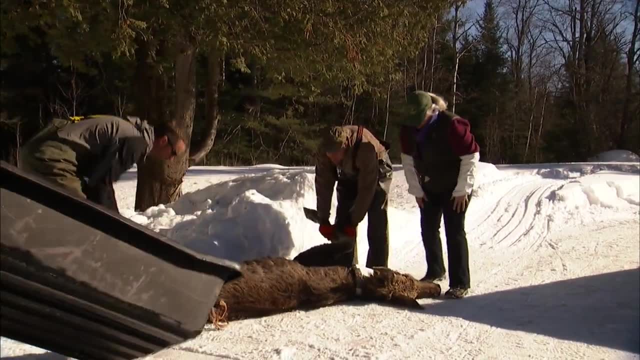 Just roll her out. The main theory New Hampshire researchers are pursuing is that the massive moose die-off is caused primarily by a devastating parasite, the winter tick. On the day we visited, biologists retrieved a dead calf that was completely covered with winter ticks. 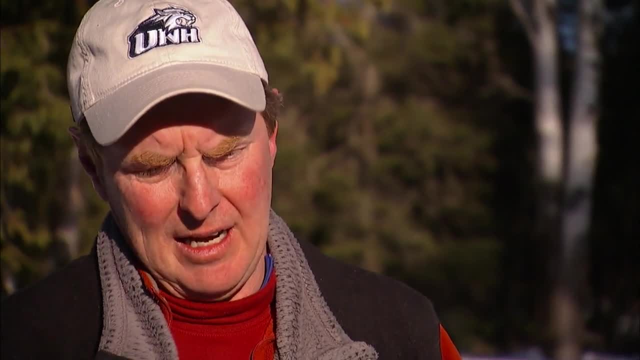 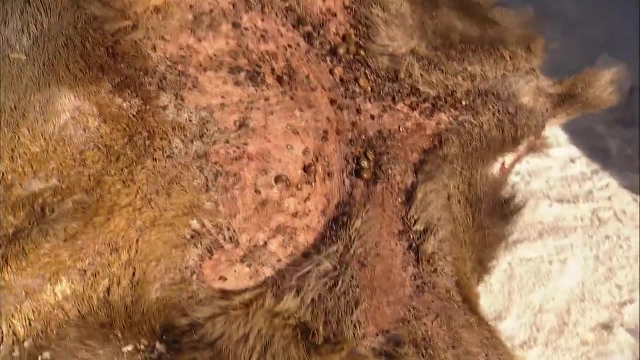 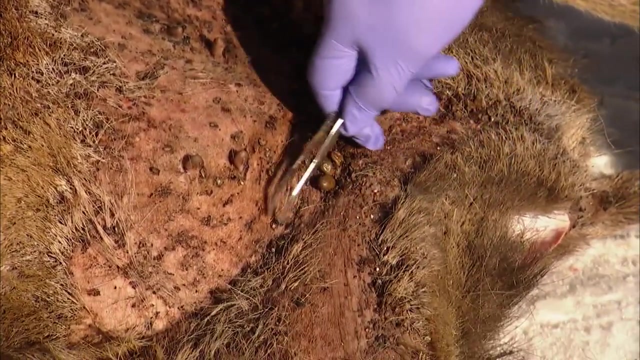 Literally, this is the walking dead. The animal is totally emaciated and there's no way it can survive. These are the engorged adult ticks. It's suspected the ticks latch on in, fall and live off the animal's blood for months. They are literally being sucked dry of blood so they can't consume protein to replace the blood loss. Their only choice is to catabolize their own tissues, and that's going to be their muscles. The hind legs on a moose are some of the most powerful legs in North America. 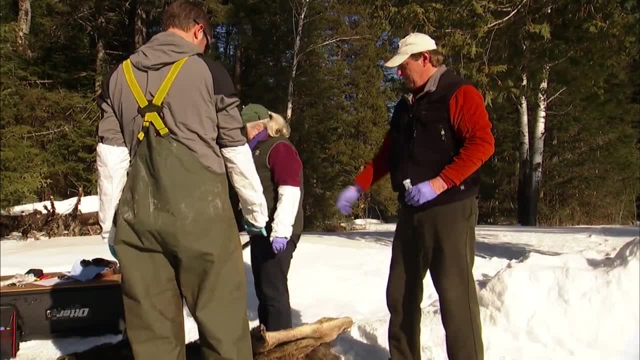 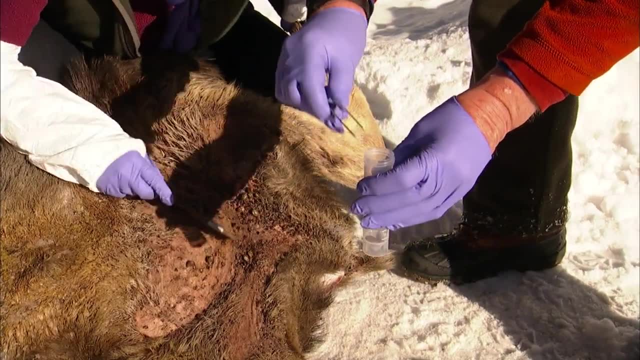 and that animal doesn't have any And it's because it's chewed up its own body to survive as long as it can. And you can see that that's quite a bit of blood. The winter tick parasite is not new, but its explosive population growth is Reaching an animal like this calf soon. 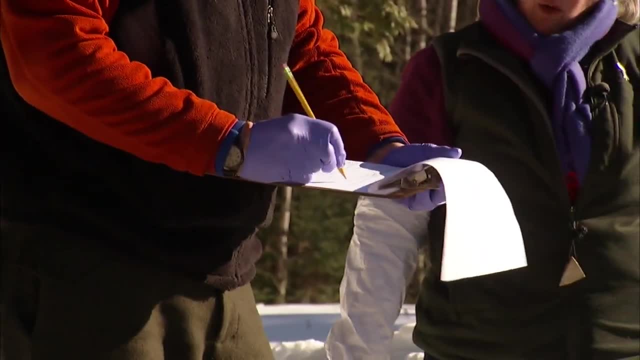 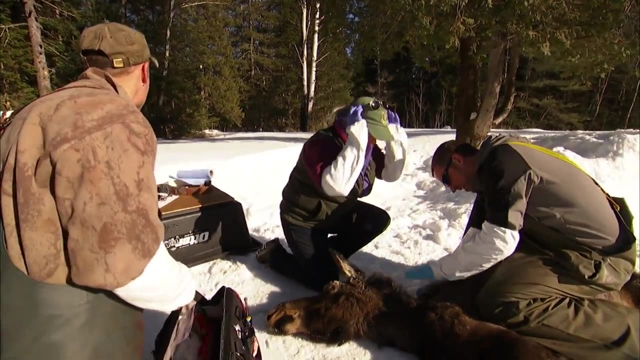 after death allows scientists to document just how many ticks there were before they drop off in pursuit of a live host. Scientists suspect that warmer winter temperatures are leading to the increased number of parasites. Shorter winters, both on the spring and fall end, play to the advantage of the.